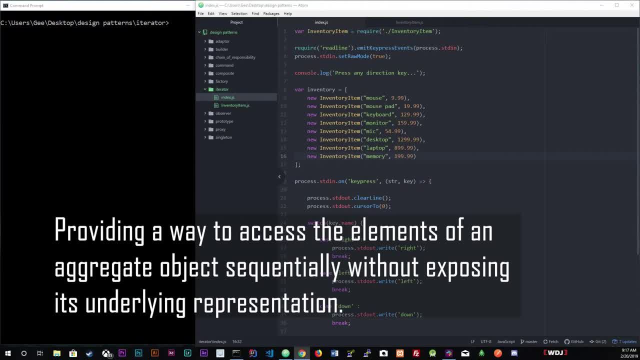 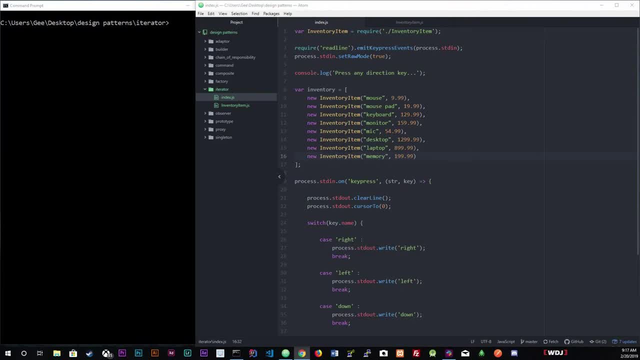 aggregate object sequentially without exposing its underlying representation. Now, the underlying representation means stacks, lists, trees, arrays. It doesn't really matter any kind of collection or data structure. That's what it means with underlying representation. And now for the overall summary. it basically means that you could traverse elements of a 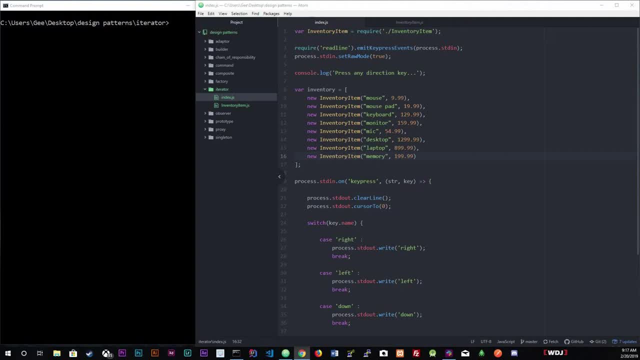 collection meaning go forward, backwards, up and down a list, free I guess. Freely, I guess You can move it around without you know what I mean. You know what I mean. So let's go into the code and I'm going to show you a pretty simple code. 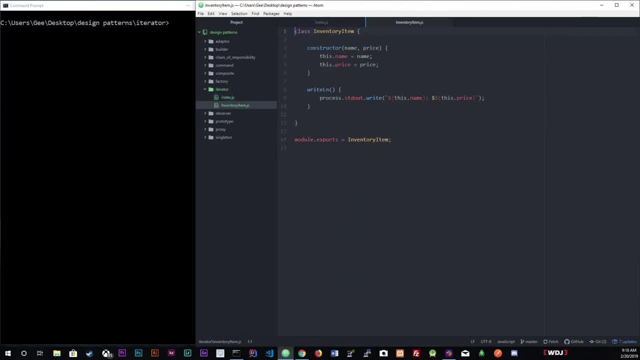 So I have an inventory list item or class, inventory item class which basically has a name and a price and is going to give us a standard output of the name and the price. I mean, this is a pretty simple class. The index is where it gets pretty interesting Now. 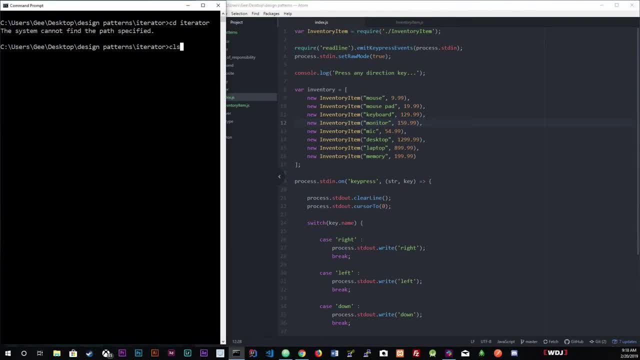 if I run this right now, nope, nope. If I run it, if I press up, it's going to tell me up. If I press right, tell me right, left, left, down, down, you know. So it was actually overriding. 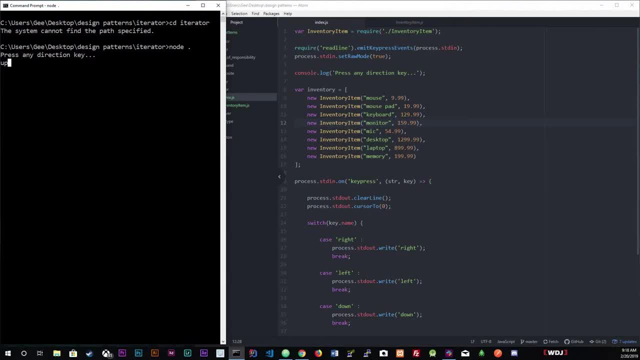 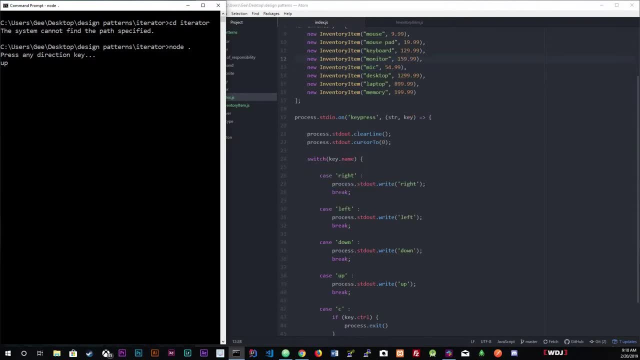 what you see on the terminal. It's not a console log, it's actually a standard output which completely takes over of what you had in the console. So- and I'm not going to, I mean you can look at this code and pretty much. 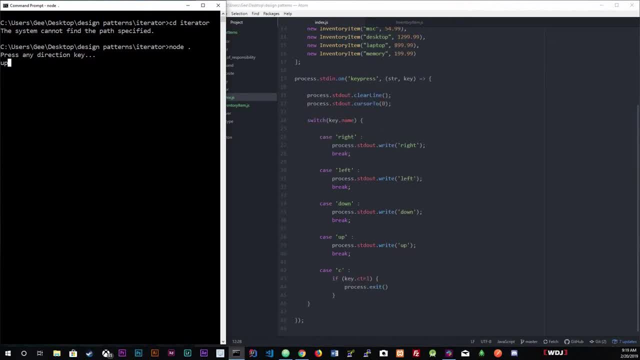 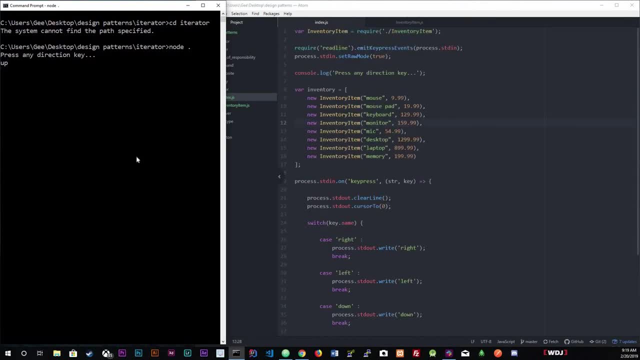 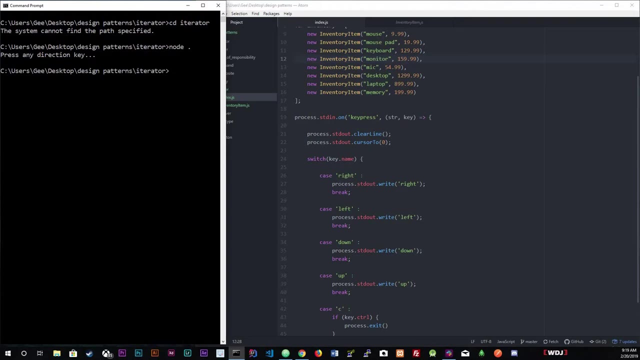 figure it out. So I'm not going to go over what I wrote here, but the pro. the point is in here. this is where we're going to create our iterator, So let me just get rid of get out of this And right here, instead of, you know, writing out the right or the actual direction we're pressing. 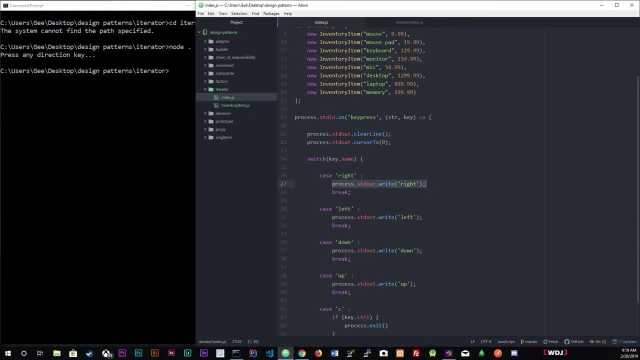 the keys. We're going to actually go into it and we all know how to iterate through an array and whatnot And you can actually do this. You know you could actually probably code out. If you press left, you can get the element of the array here. If you press left, get the previous element that. 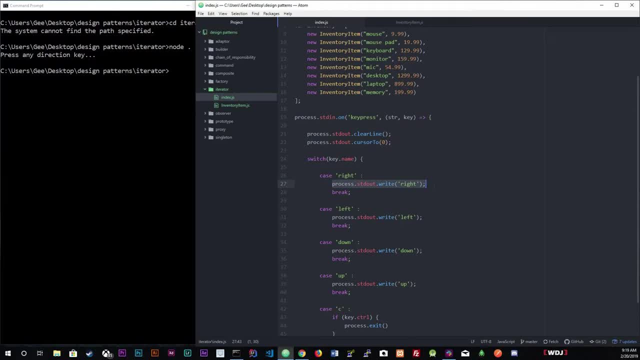 from that array. But the thing is, the iterator is meant to be used for different collections. It has an interface that would do it for different collections. You know what I'm talking about. So if I did decide to do it with the array right here, right, getting the array to the right, well, 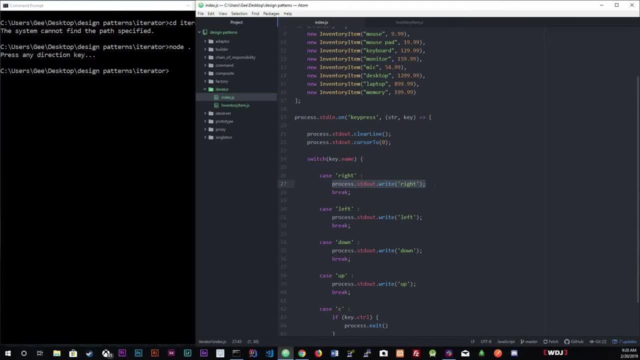 let's say that you want to get it the right, or the next element of a tree. Well, right now, writing an array code is not going to be the same as writing for the tree right? So this is why we have an interface. So, in here, instead of doing writing out the right, we're going to actually 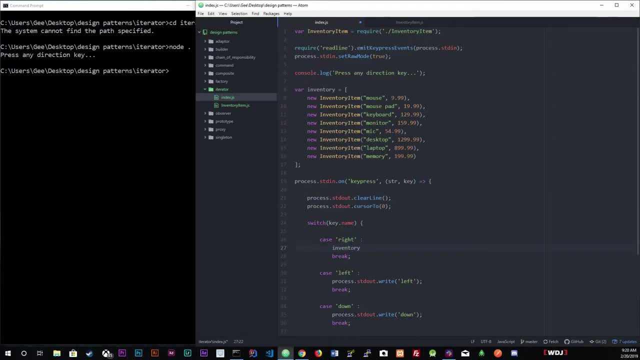 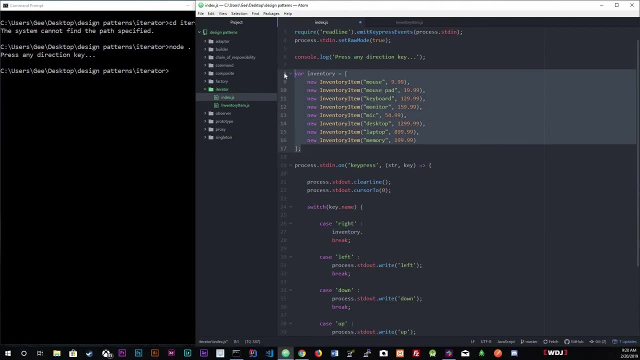 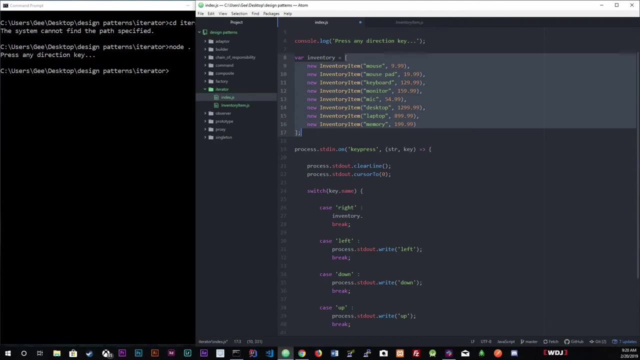 go to the inventory which is our up here, our array of stuff And we're just going to- or right now it's an array, right, But it's, I'm going to say- a collection. This could have been a tree, It could have been a stack, It could have been all sorts of things, but 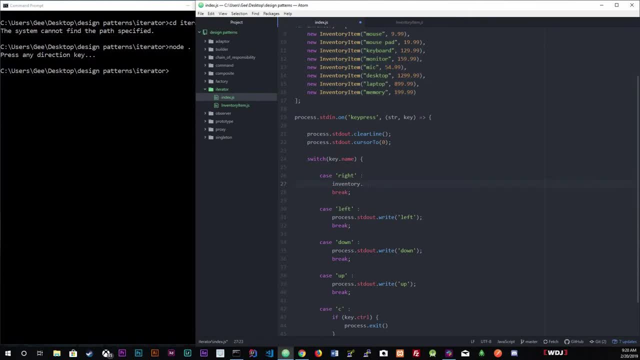 I just decided array for simplicity. So we're going to do inventory dot next, We're going to call next and we're going to do and call out the method that we have in here, which is right line, Okay, Right line, just like that. And we're going to actually grab this line and we're 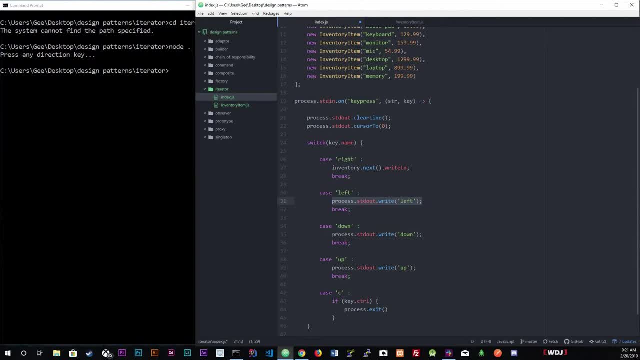 going to do it for here as well. I'm going to do it right here as well, And right here. Oops, Boom, Okay And paste. Now we're going to do it for the right, We're grabbing the next. for the left, we're going to grab the preview. Okay, What am I doing here, Eve? Okay, 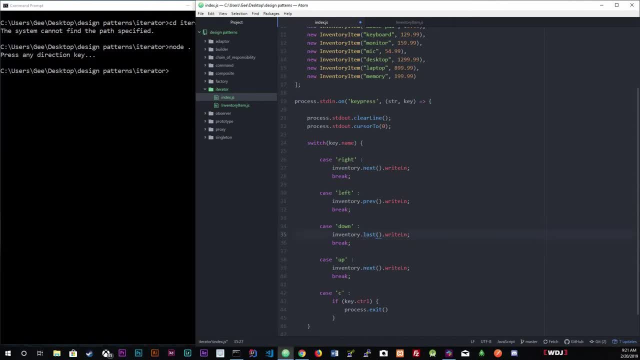 And right here we're going to get last, and when we do the up key we're going to get the first element of the array. So this is pretty much simple stuff, guys, Control save. now we're going to go into our inventory item right here and actually start, uh, adding all the 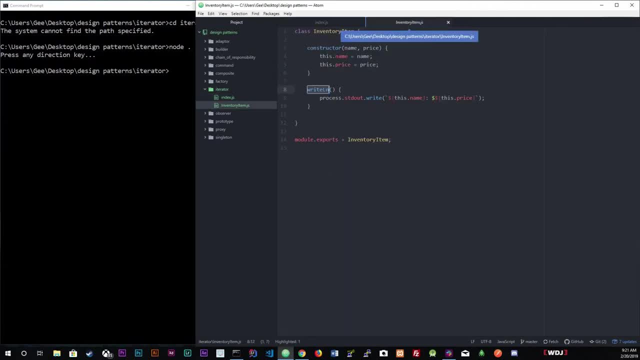 methods that we added here, which is the next pre blast and first scratch, that we're not going. we're not going to be, uh, doing it in the inventory item. we're going, we're going to be doing it in a different file. so up here we're going to create a new file require, uh, dude, where's my comment there? 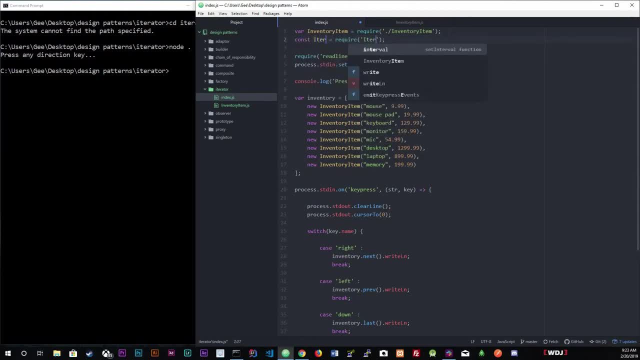 it is okay, we're going to call it the iterator. i'm sorry, guys. i was looking at my notes and i was like, yep, i need my. i forgot this one thing up here and actually in here, instead of, uh, just assigning this inventory and array, we're going to assign 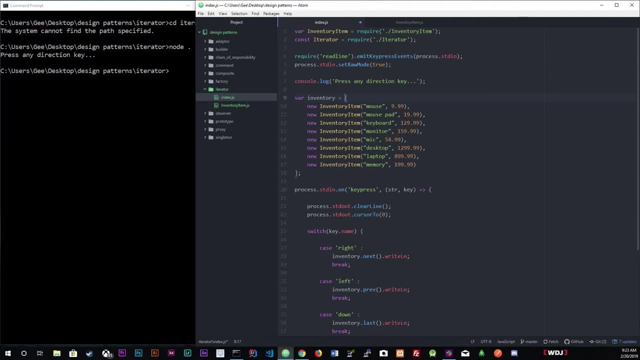 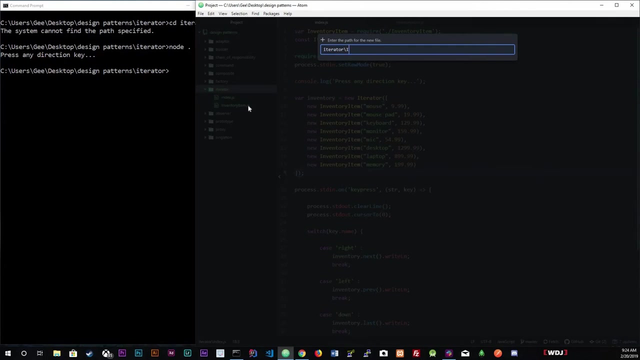 inventory a, a new instance of this iterator and passing in the array or the collection inside the iterator. so new iterator, and we're going to just pass it in the array. that's it. and then now we could actually create another file called the iterator. so new file: iteratorjs. 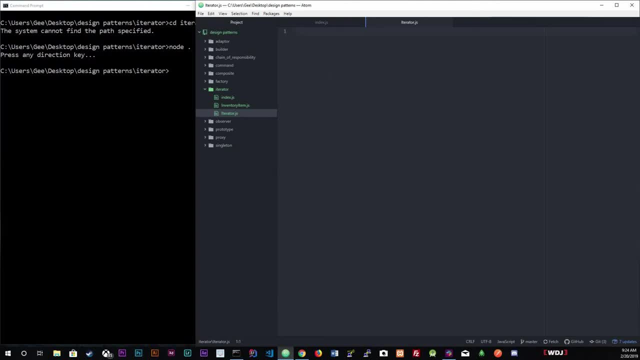 and in here, this is where we're going to actually do our our uh iterator. so let's do a class, call it iterator and we're going to export this. so module dot exports is going to equal iterator uh-huh. and then inside of here we're going to get all of those. 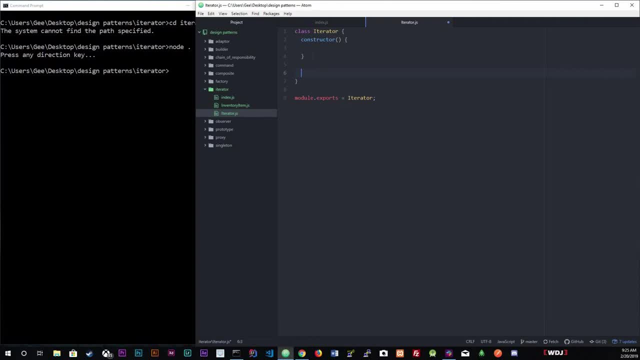 um, methods, right, so we're going to have our next, our prev, oops, our last and our first. now these, uh iterators, you typically have a has next kind of method, so has next. and then you also have the current right, although we don't call these, but you typically do have it because you do. 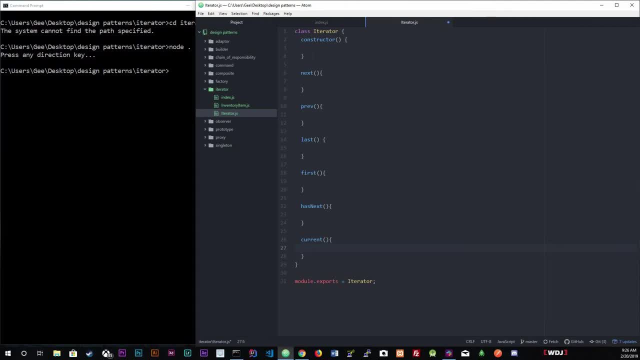 want to know what you're currently on or if it does have a next. so we're going to go start with the constructor, and the constructor does take, uh, an array. so i'm just call it items and if we don't pass in something i'm just going to pass in, i'm going to default it to an empty. 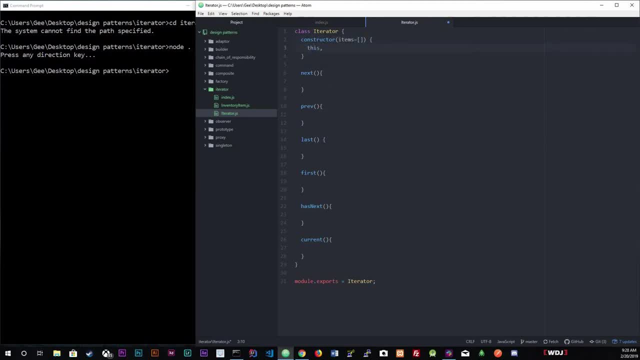 array, and then we're going to say: this dot index, we're going to set that to zero, because we want to start off with zero for our first index, um, and then this dot items is going to equal items. okay, now let's, let's start with our first, first of all, down here. um, obviously we're going to return. 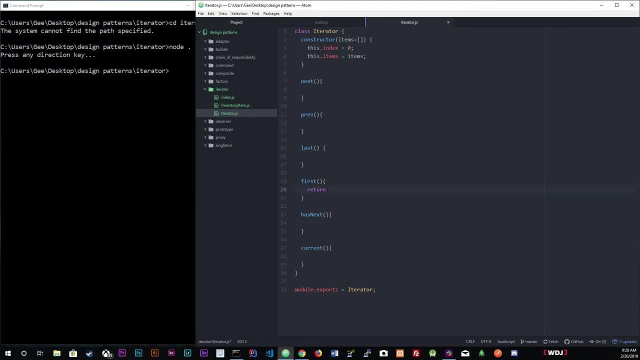 we could do it a simple way. i'm pretty sure you know that you could do it this: dot items and then return the first first item or element in the arrays list. right, but their javascript actually gives us a pretty cool way of doing this and we're going to actually assign it. 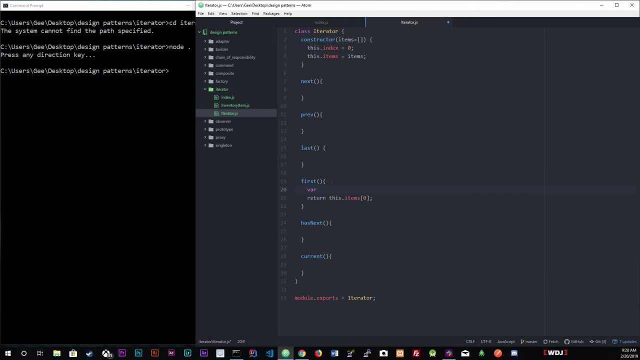 var. we're going to destruct their destructure. the first item first, just like that, and this is going to and pass in this dot items and this will give us the first uh element inside the array, which is pretty cool. um, obviously, if you wanted the second one, you could have done like, second, like. 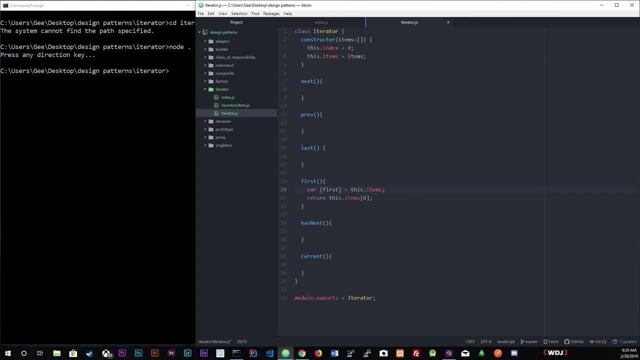 this, but we just want the first one and we're going to just return first. that's pretty cool. i'm just. i'm just laughing because if you look at this for for a very long time, you start thinking, well, this is how i think i'm not too sure very with this is, but you start thinking that this is. 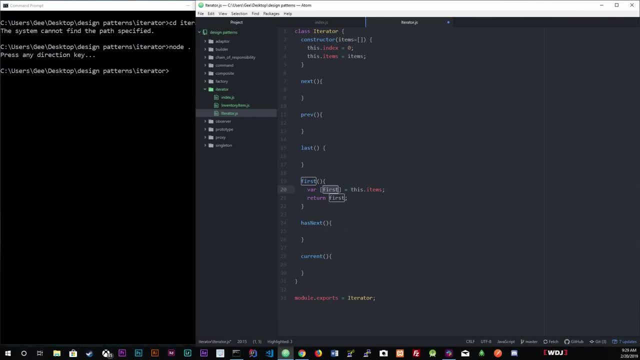 um, it starts looking weird, the words i'm not, i'm not, i'm not too sure. anyways, we could do the same thing with last, so we can actually destructure this, so we can actually copy this right here, right, but instead of getting the first one like this, we're going to actually have to reverse the. 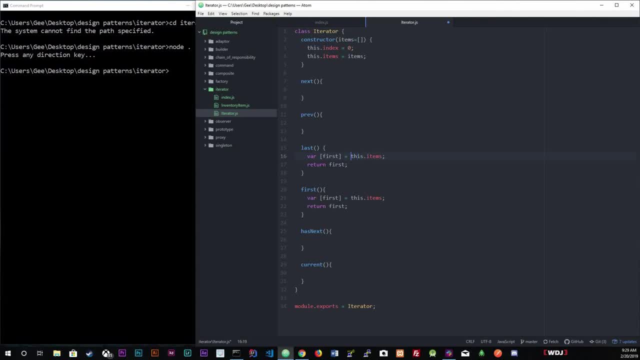 array, so dot. i'm going to just do this so that way we make a copy. it's not a good idea to actually manipulate the original array. we want to make a copy of the array, so i'm actually set this in brackets and use a spread operator to copy this: this dot items, and then we're going to reverse. 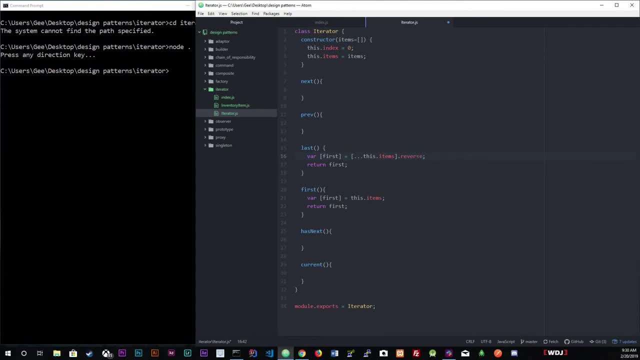 the array. so that way, now it's reversed and we're going to grab the last. it's going to be called the last item and last row save, which is pretty cool. it just gives you a new way of actually doing things. um, you know, so you're welcome. um, going on to current, the current is going to be pretty simple: return this dot items. 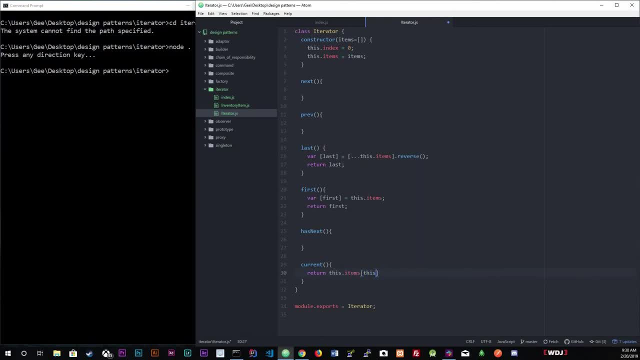 and this dot index. whatever index we're in, we're going to return that. so we're on. zero is going to return the first one. obviously, whatever index we're in, we're going to return that. let's go ahead and do that. let's go to has next. all right, for has next, we're going to return. 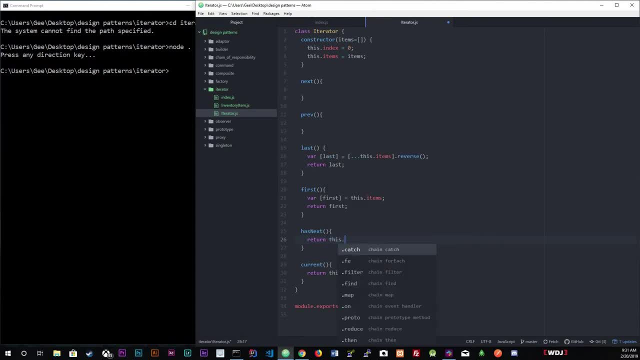 this dot index. if it's less than this dot items, dot length, negative one minus one. i mean just like that. so this is gonna, oh, not like that, like this. so this is going to return if it does actually have the next item. so if it doesn't equal a negative one, which means it's reached the end of the array, then we're okay. 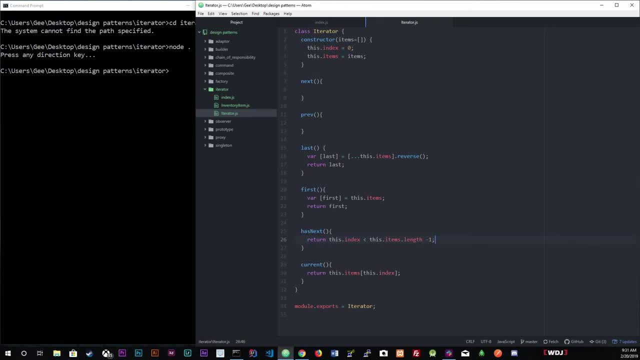 um, not going to the pre, or we could actually do next, next. now for the next. we do have to check if this dot has next. that's why we have the has next method right here. um, or this is one of the reasons why you would want to use has next. 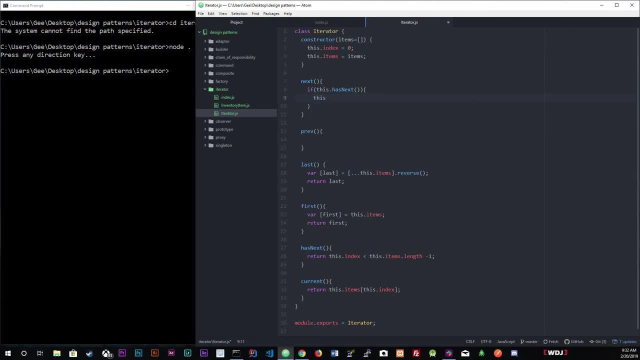 We're going to check that. If it does, then great, We're going to do. thisindex plus equals 1.. We're going to just add a 1 to that index And then we're going to return thiscurrent- And I spelled current- right. 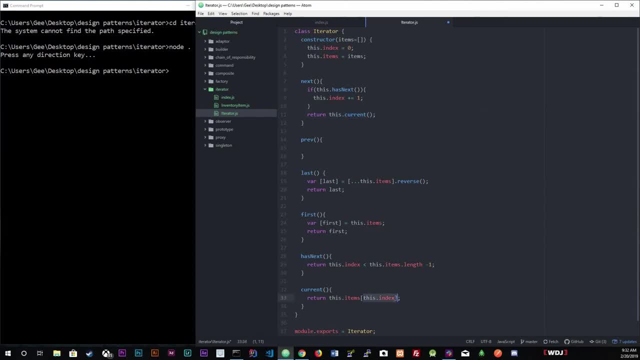 And you'll see, remember, current is going to return, whatever the index is which we just incremented here, And this is why we're calling current. Now, going to the brief, we do have to check again. So if thisindex does not equal 0, if it does equal 0,, obviously you're in the first element. 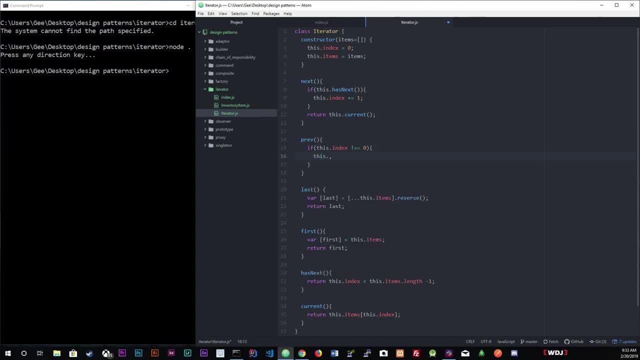 in the array. So We're going to do thisindex and we're going to just decrement it by 1, minus equals 1., Just like that. And we're going to return thiscurrent again, And I didn't do the return statement in front, so return thiscurrent Control-Save. 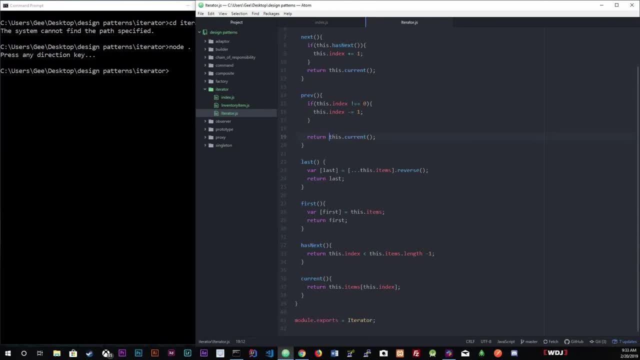 So this is our iterator class, which we- I mean, you know it's pretty simple stuff, guys, But this is how you would do it. You would, if you had another data structure, you would include it in here. You know, you'd probably use the type of: if it's an array, then do it this way. 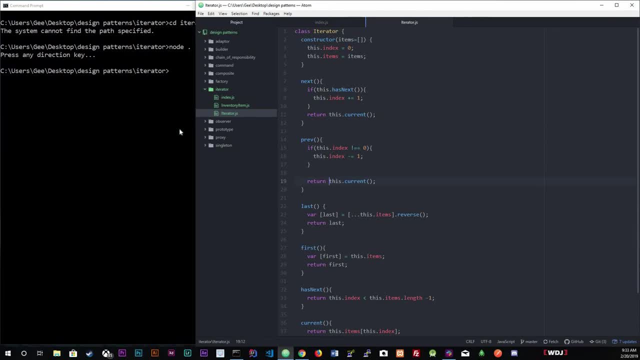 If it's a tree, then do it this way, you know. But it's pretty simple. I'm like guys, I'm telling you this is a pretty simple one. Now, if we actually run this again. oh, I forgot to do something. 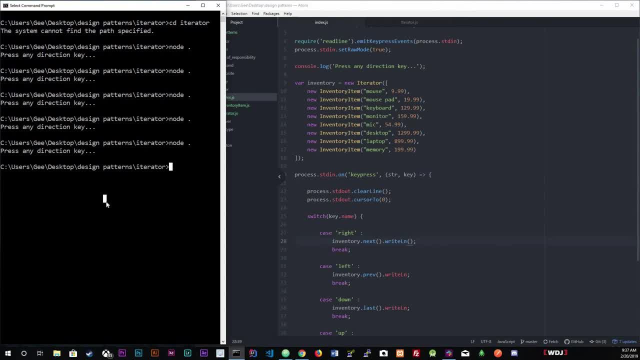 I'm so sorry, Control-C out of that. Sorry guys, I was debugging and I did forget. It's always something so hard to do. I'm sorry, Control-C out of that. Sorry guys, It's so simple. 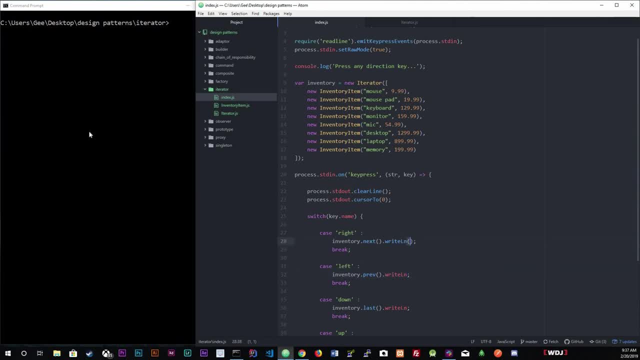 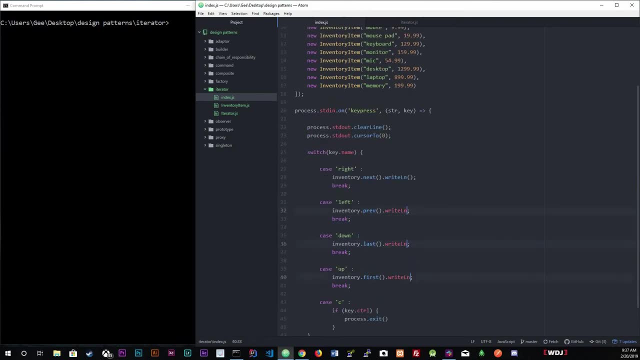 I forgot to add the parentheses b on the end of this. That's why you didn't see anything when we originally tried it. And let me just add the closing open and closing in parentheses on all of these Control-Save this Now. if we try it, press any key. 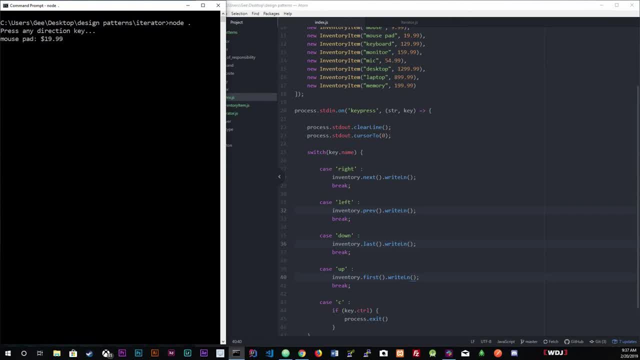 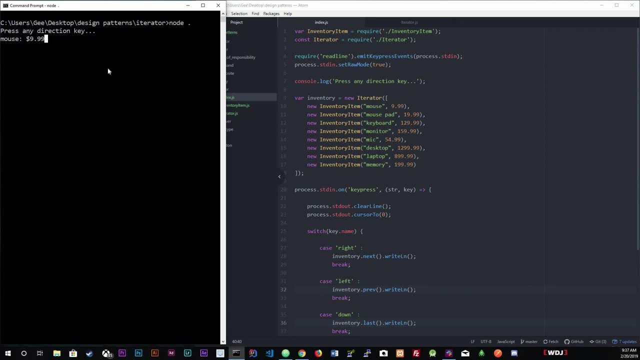 So if you go to the right, we should get the next, which you can see right here, we're grabbing the next. So mouse pad, If I go up, we get mouse, which is our first item, Or if I go down, we get memory, which is yes. 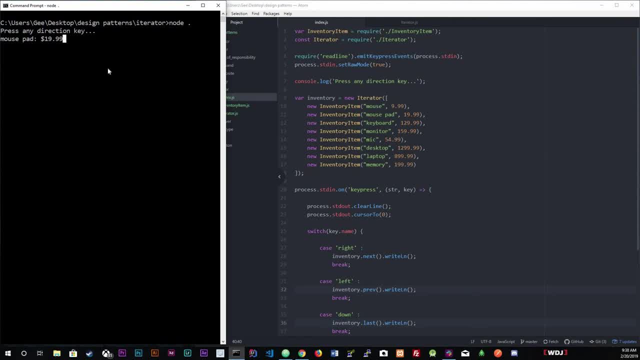 If I go to the left, we should get mouse pad. It's going to be the last. whatever we had, last Keyboard monitor, mic, desktop, laptop memory, And we can't go to the right no more. so let's go back. 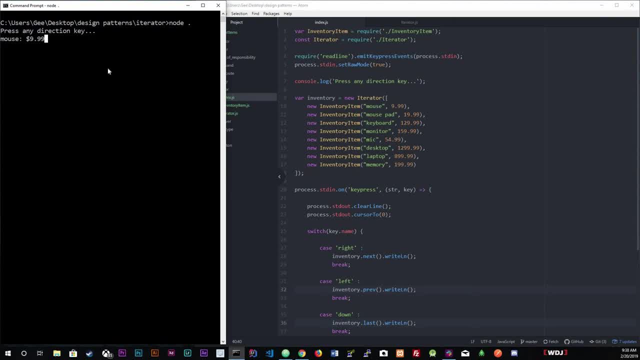 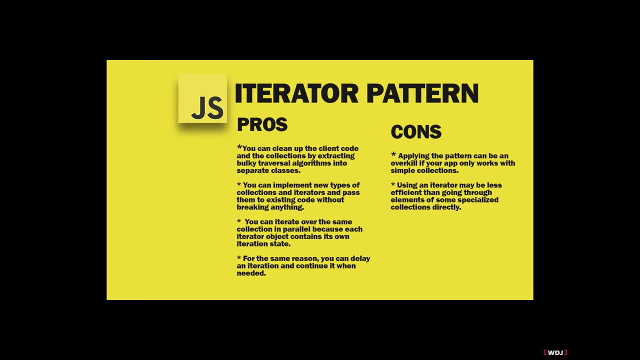 Laptop desktop mic down up, down up. It's pretty cool. But yeah, that's the iterator pattern, guys. So let's go straight to the pros and cons and when and where you would use this. So let me actually provide you a quick summary of what an iterator is supposed to do. 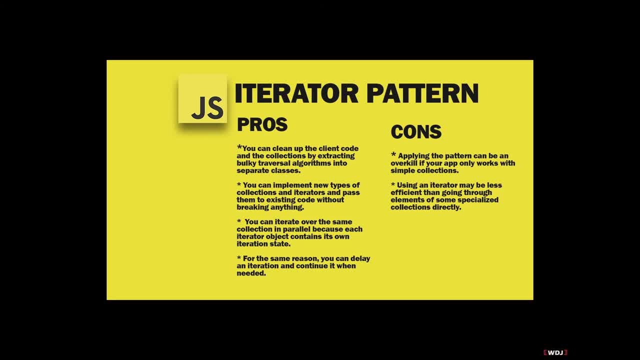 So it's supposed to provide a uniform interface to actually iterate through any collection available. So that's basically what it is: a simple interface that you could just dump into any collection. dump that into the interface and it'll iterate through everything. That's basically what it is, guys. 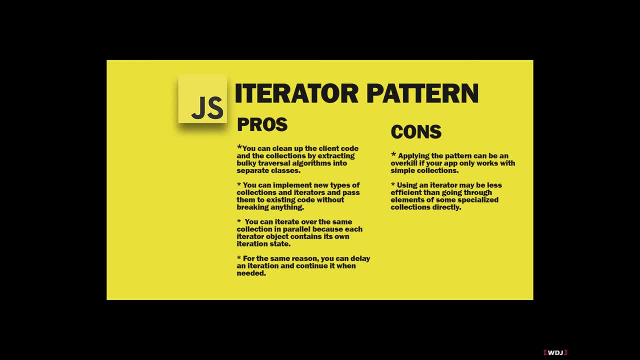 So let's go for the pros and cons. The pros and cons: You can clean up the client code and the collection by extracting bulky transversal algorithms into separate classes. You can implement new types of collections and iterators and pass them to existing code without breaking anything. 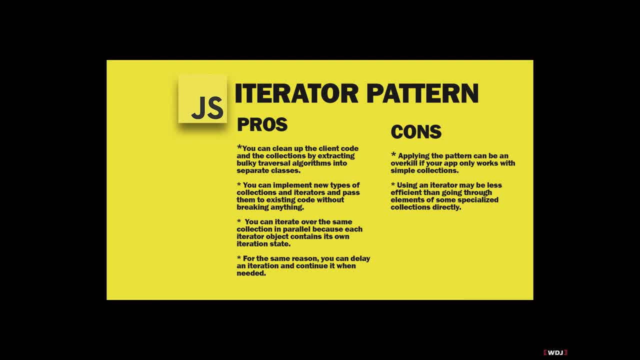 You can iterate over the same collection in parallel, because each iterator object contains its own iterator state, Like we've done. like in the code, we did have that new new iterator. We're creating an instance of that iterator. You could create multiple instances. 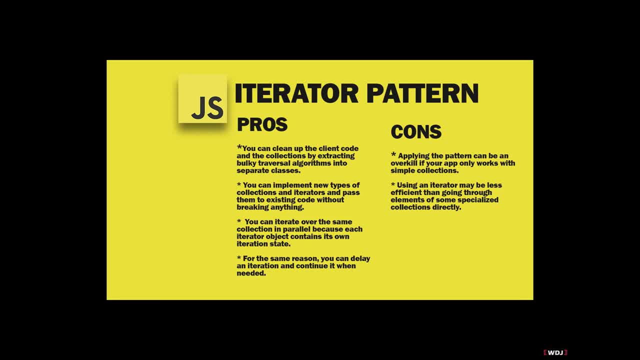 and every instance is going to have their own index. Yeah, so you can loop through multiple collections, if you wanted to, in the same application and it'll iterate the way as expected. And for that same reason, you can delay an iteration and continue it when needed, which is a pretty cool thing. 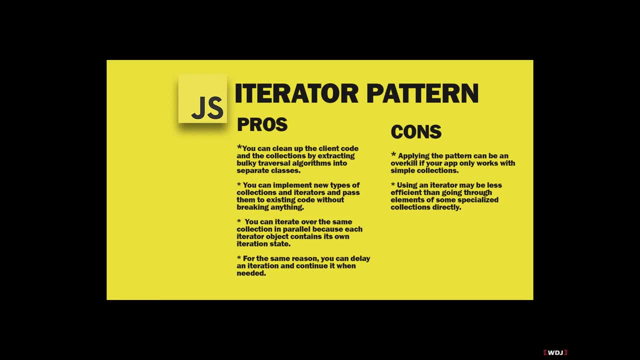 So for the cons, Applying the pattern can be an overkill if your app only works with simple collections. obviously I thought that I needed to add that in because you will, I guess, just by learning something new, you want to incorporate it. 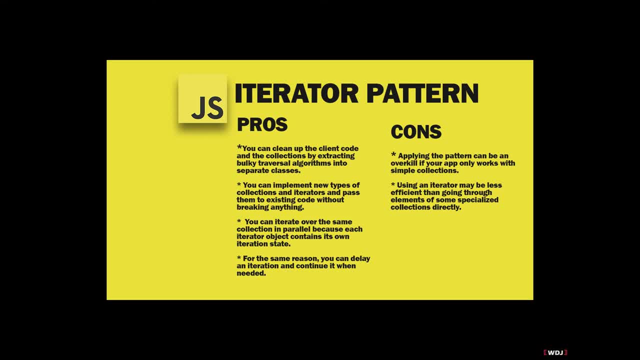 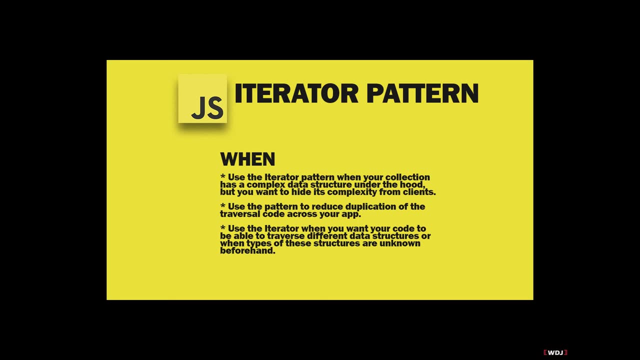 But if it's a simple application, don't do it. Using an iterator may be less efficient than going through elements of some specialized collections directly. So that's another con. All right, Let's go to the wins. So the wins: Use the iterator pattern when your collection has a complex data. 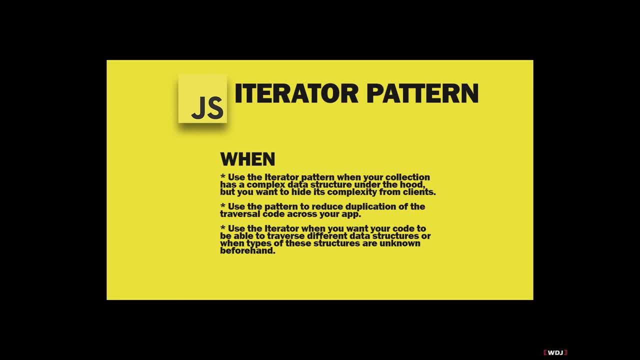 structure under the hood, but you want to hide its complexity from clients. So either for convenience or for security reasons. So a little bit about this. The iterator encapsulates the details of working with a complex data structure, providing the client with several simple methods. 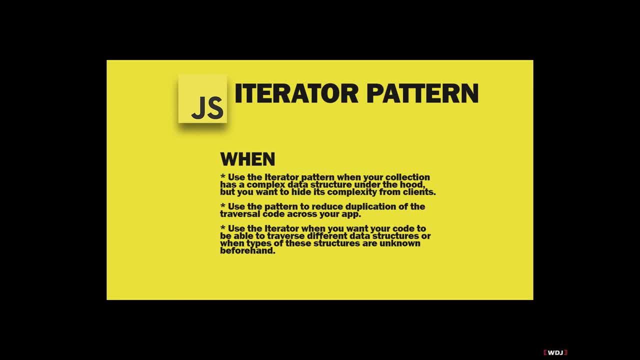 of accessing the collection elements. While this approach is very convenient for the client, it also protects the collection from careless or malicious actions which the client would be able to perform if working with the collection directly. So that's why we said for either convenience or security reasons. 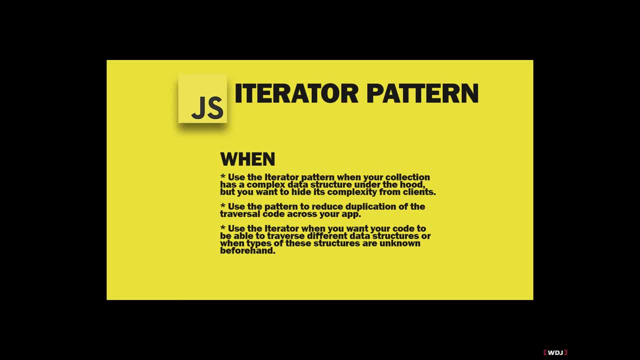 Use a pattern to reduce duplication of the transversal code across your app. So the code of a non-trivial iteration algorithm tends to be a very bulky one. So when it's placed within the current collection it can't be used as a temporary code. 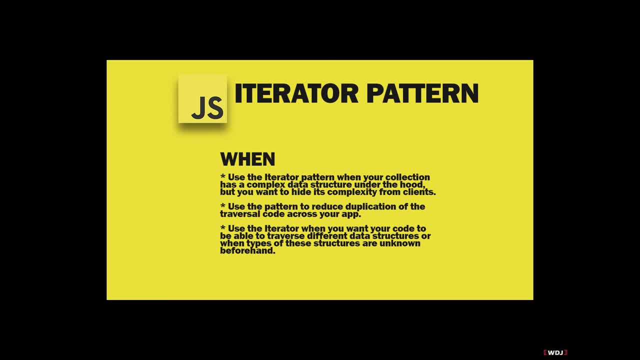 business logic of an app, it may blur the responsibility of the original code and make it less maintainable. so by moving the transversal code to a designated iterator, it can help you make the code of an application more lean and clean. lean and clean- i didn't even